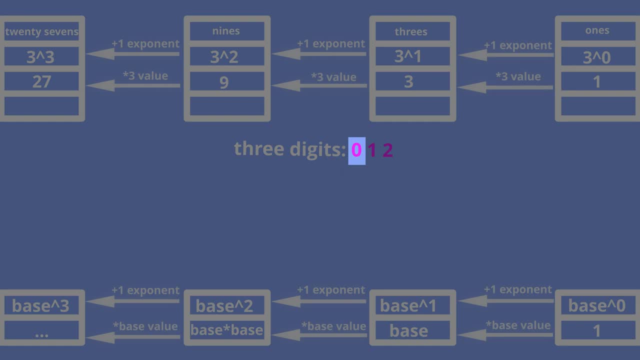 Please pay attention that 0 is the first digit and the last digit equals the base minus 1, so in our case, 2 equals 3 minus 1.. Please pay attention that the number of digits equals the base. In our case, base is 3, and the number of digits is 3.. 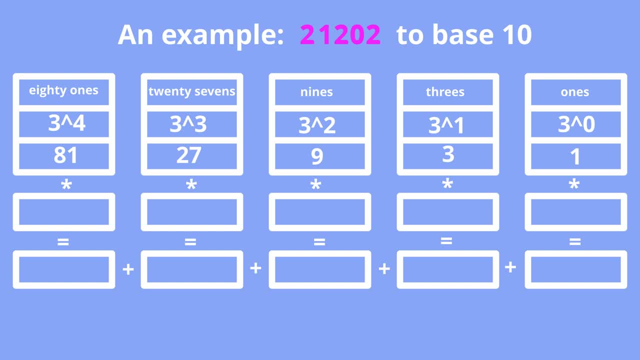 Let's, for example, convert 2, 1, 2, 0, 2 from the base 3 number system to the base 10 number system. First we arrange from right to left all digits in corresponding positions. Then we multiply digits by the weights of corresponding positions. 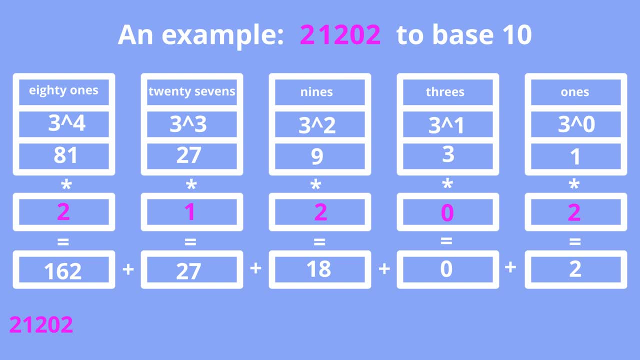 and sum up intermediate results. So 2, 1, 2, 0, 2 equals 2 times 81 plus 1 times 27, plus 2 times 9 plus 0 times 3 plus 2 times 1 and equals 209.. Now let's, for example, convert the number 65 from the: 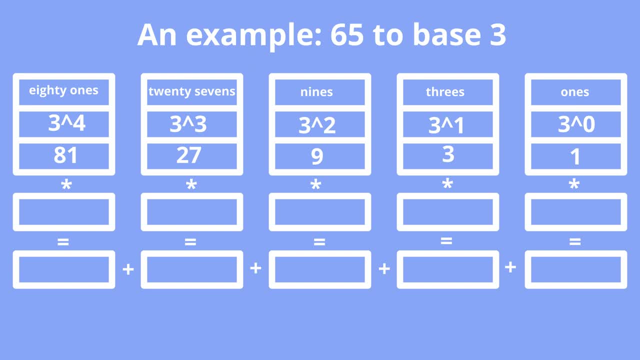 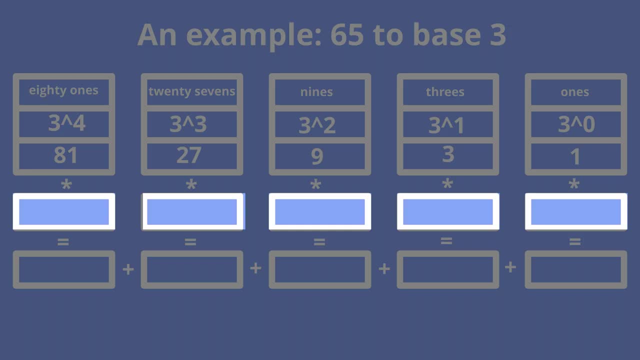 base 10 number system to the base 3 number system. To do this, we need to fill with digits 0,, 1 and 2 these positions in such a way that the sum of these positions will give us 65. We don't need to try all possible variants of 0s,1s and 2s. We can move from left to right. 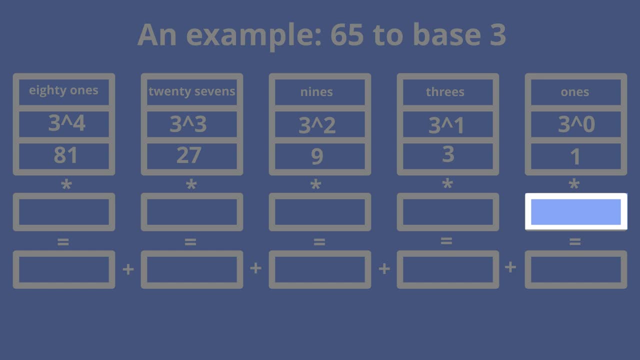 each time trying to fill a position with the maximum digit. Since this is the base 3 number system, the maximum digit is 2.. If, in some step, the sum of the product of digits that were already taken and corresponding weights is greater than the target number, we need to decrease the digit by one. in the base three number system. 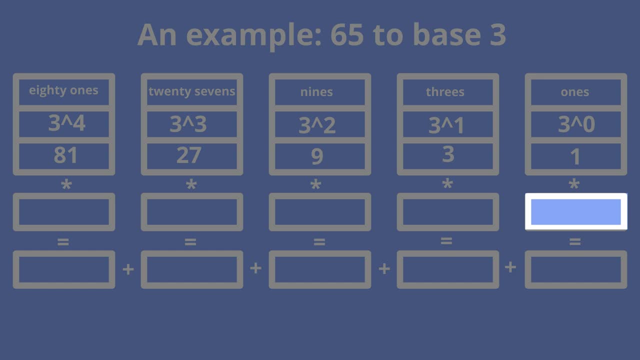 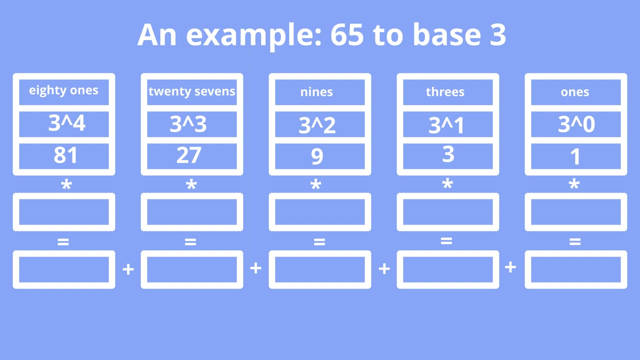 from two to one and if it will not be sufficient, decrease from one to zero and then continue the same steps till the extreme right position. as the starting position, we will take the position of 27s, because the weight of the next to the left position of 81s is too great. so 65 equals, let's. 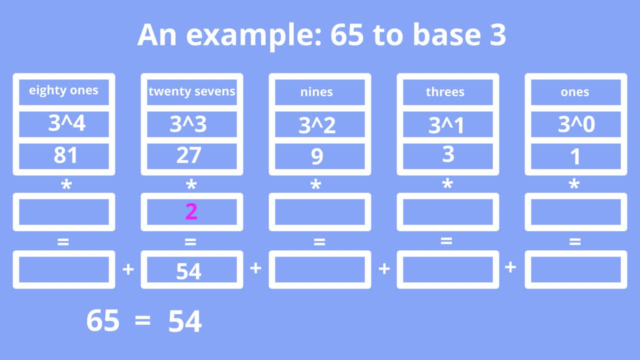 put digit 2 in the 27s position: 27 times 2 equals 54. 54 is less than 65, so we can continue. let's try to put digit 2 in the 9s position now: 9 times 2 equals 18, 54 plus 18 equals 72, which is greater than 65. so let's decrease by one digit. 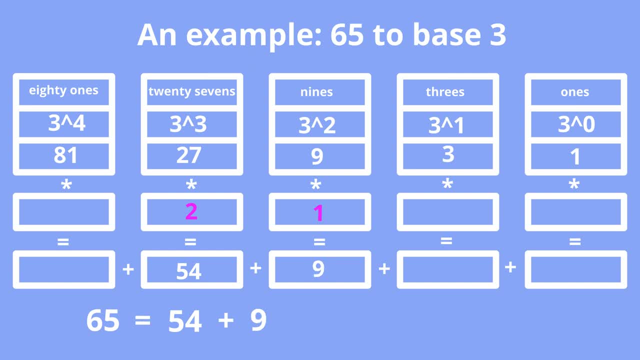 in the 9s position down to 1. 54 plus 9 equals 63, which is less than 65. so we can continue. let's try to put digit 2 in the 3s position: 3 times 2 equals 6, 54 plus 9 plus 6 equals 69, which is greater than 65. so let's decrease by one. 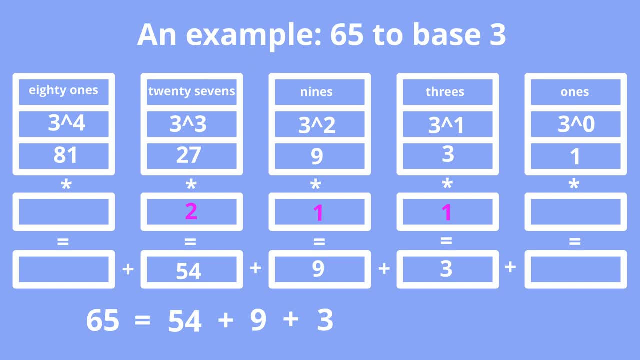 digit in the 3's position down to 1.. 54 plus 9 plus 3 equals 66,, which is greater than 65. So let's decrease by 1 digit in the 3's position down to 0.. Next let's put digit 2. 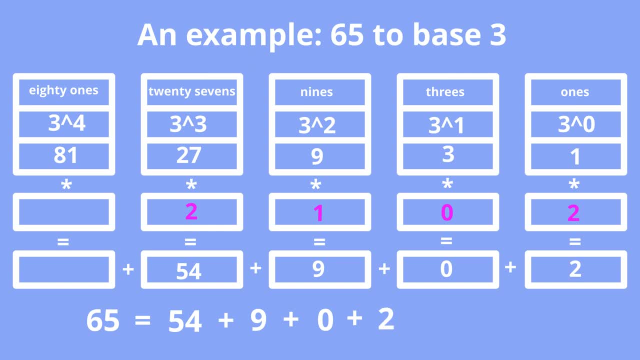 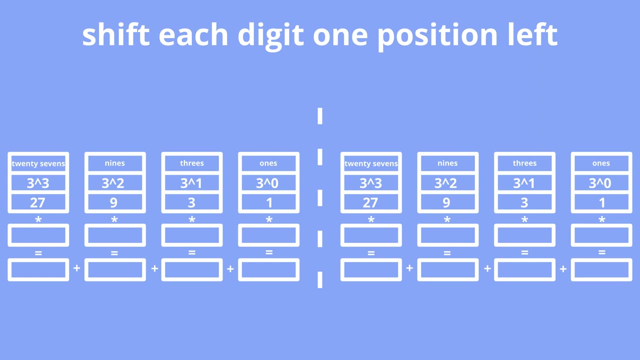 in the 1's position, 54 plus 9 plus 0 plus 2 equals 65. We obtain the required result. Now let's consider shifting each digit one position to the left. This is equivalent to writing 0 to the right of the number in any positional number system And, as a result, 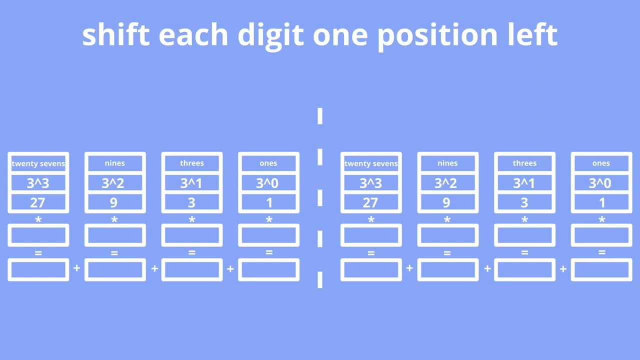 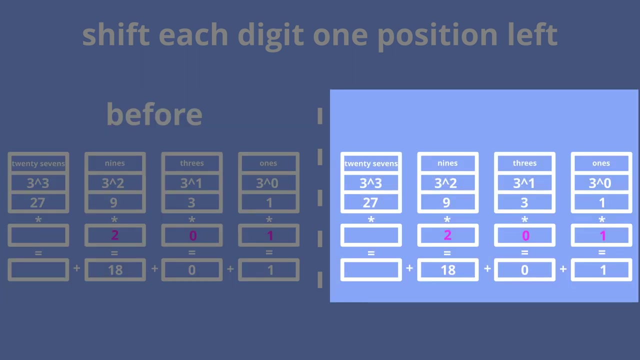 the number will be base times greater. So in the base-3 number system it will increase 3 times. Let's consider an example of left shifting number 2,, 0, 1 in the base-3 number system On the left is the number before the shifting and on the right will be the number in process.